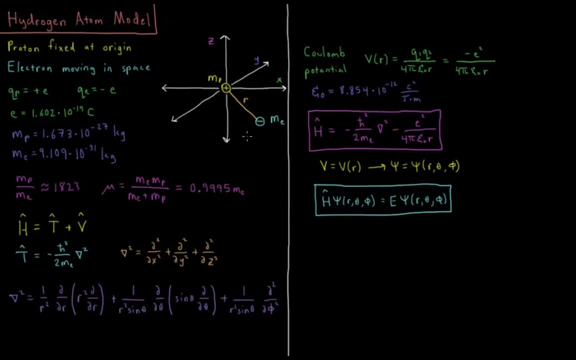 will just move much, much faster, having a similar kind of charge but a much smaller mass. And then we also look at the reduced mass of this system, and we can justify this as well. the reduced mass when you have one that weighs about 2,000 times more than the other. 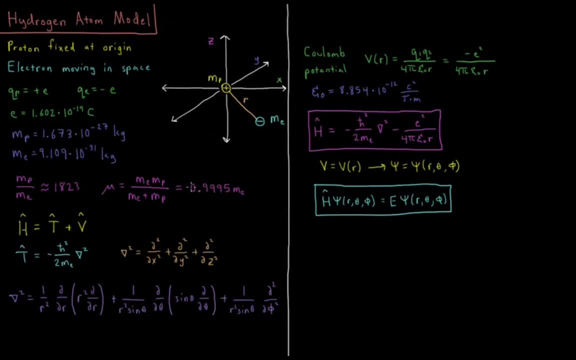 As we saw in the Rydberg formula example, is 0.9995 times the mass of the electron. So the mass that we're using is almost exactly equal to the mass of the electron. And if we go ahead and just say our proton is fixed at the origin, then we can just go ahead and use mass of the. 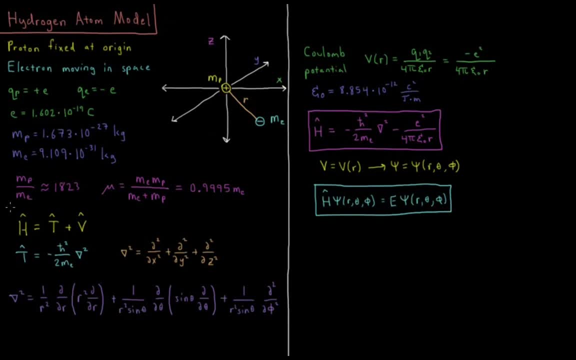 electron Instead of this reduced mass. Okay, so in order to solve for the wave functions and energies of this hydrogen atom model, we need to define our Hamiltonian operator. So the Hamiltonian, as in every case, is kinetic energy plus potential energy operator, So kinetic energy operator minus h bar squared over two times. 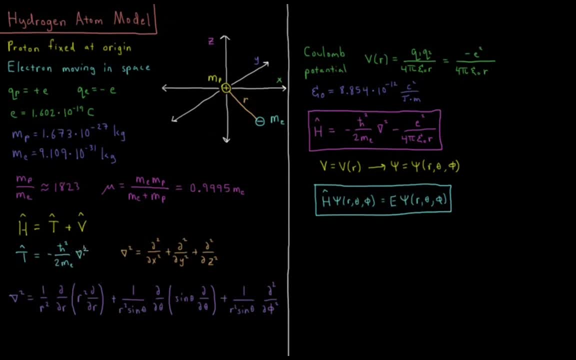 mass of the electron times del squared, del squared being the Laplacian operator In Cartesian coordinates in three dimensions. that's just the sum of the second partial derivative with respect to x, y and z. But it's more natural for us to use a wave function which is in spherical polar. 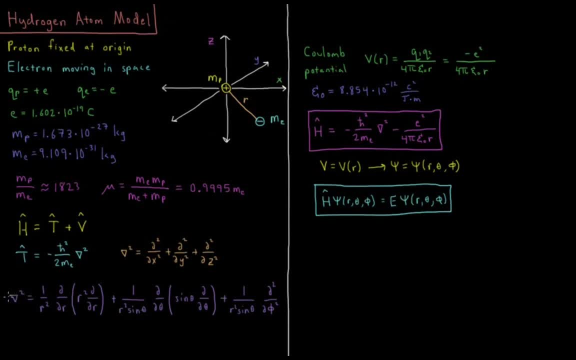 coordinates here. So our Laplacian is going to be in spherical polar as well in terms of the values r, theta and phi. So the Laplacian is much more complicated looking and spherical but it's going to be much easier to express our 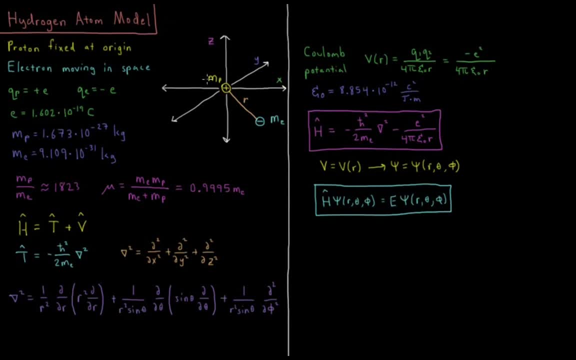 wave functions and energies in terms of r, theta and phi, rather than x, y, z. So the Laplacian is: del squared equals 1 over r squared partial with respect to r quantity, r squared d dr, plus 1 over r squared sine theta, partial with respect to theta of. 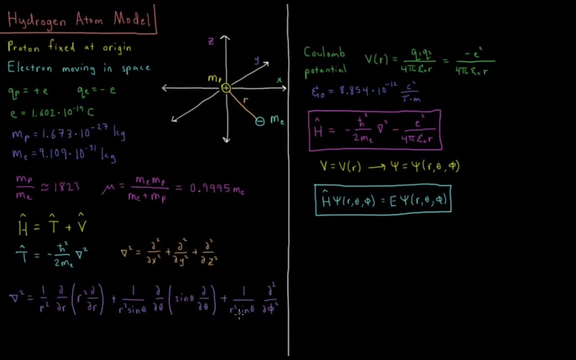 quantity sine theta d, d theta plus 1 over r squared sine theta. second derivative with respect to phi For our potential energy. our potential energy is defined by the Coulomb potential. These are both charged particles. They interact with one another through the Coulomb force and their potential energy.